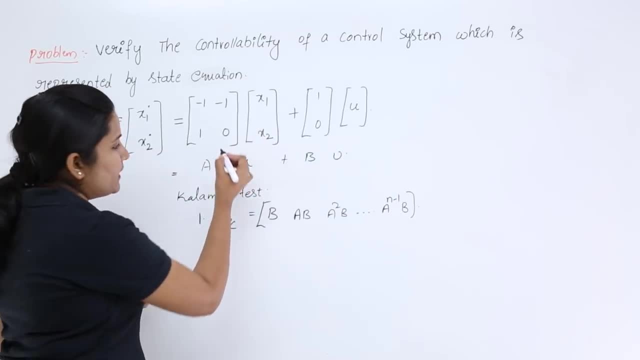 n by n matrix. here this is 2 by 2 matrix, and coming to here, this is 2 by 1 matrix. So order is equivalent to 2, n by n, n by 1, where n is equivalent to 2.. So by the given data, 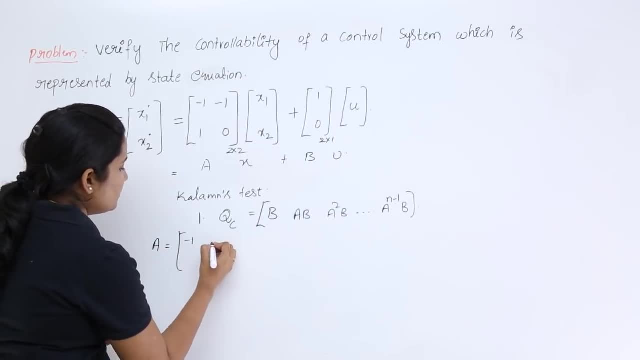 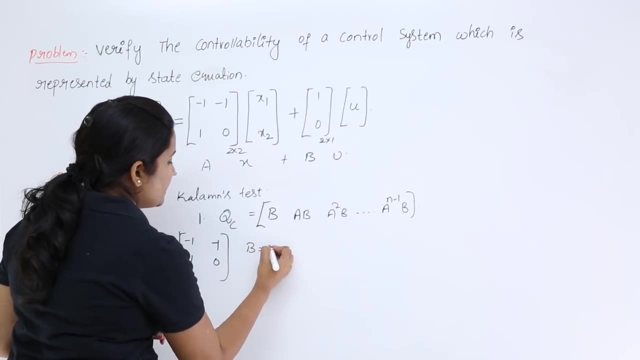 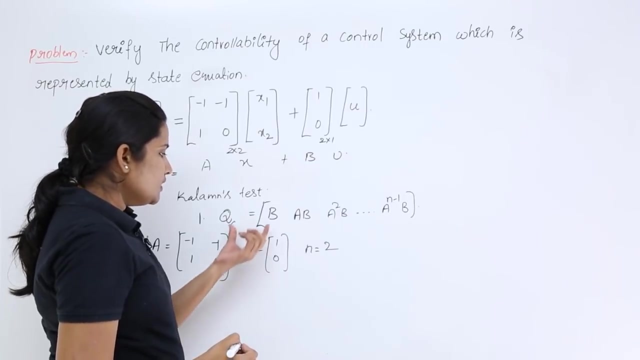 A is equivalent to minus 1, minus 1, 1, 0,. this is the given data I am writing- and B is equivalent to 1, 0 and n is equivalent to 2.. Now this matrix will become so: this is equivalent to. 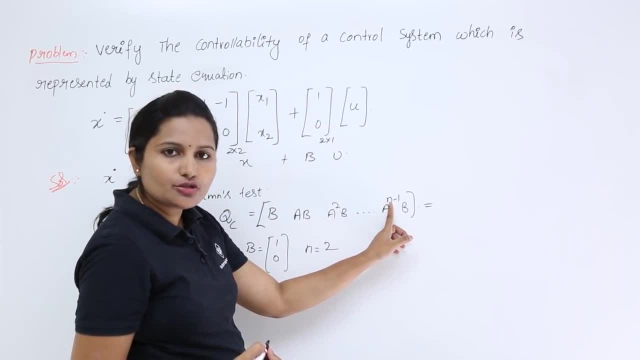 when I am taking n is equivalent to 2, this is limited to A power 2 minus 1. that means A power 1 into B Means it will limited to only 2 terms. So this matrix will be for the given data. the matrix will: 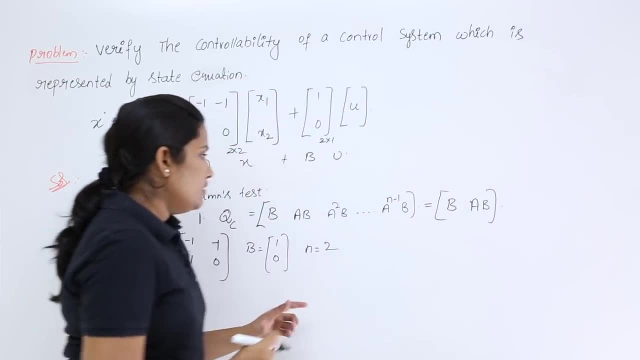 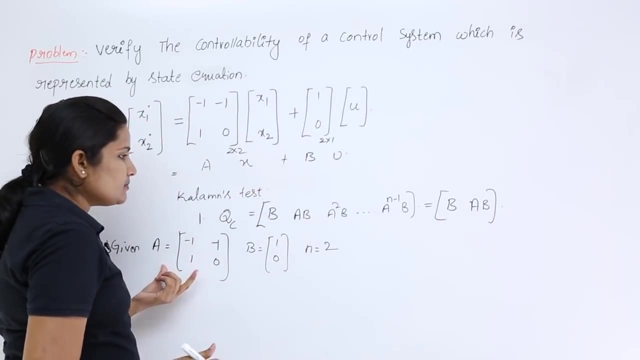 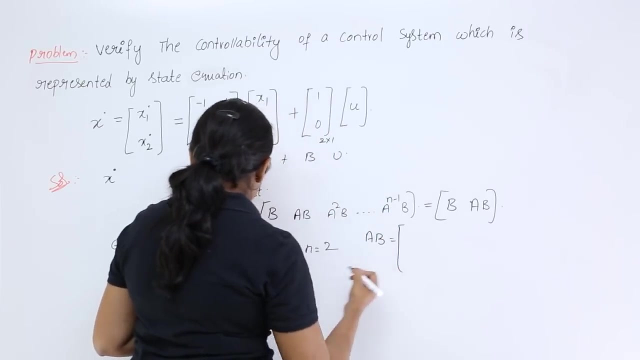 be B, A, B. So now everything available with us just to calculate A, B is needed. So here I am just multiplying A and B. A and B is equivalent to A into B is equivalent to minus 1, minus 1,. 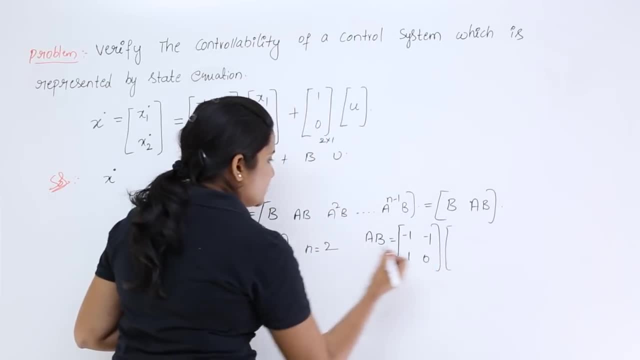 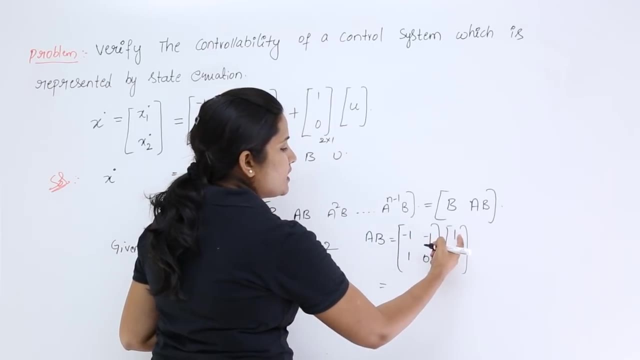 1, 0 into B. B is equivalent to 1, 0. If you multiply these 2, what you are going to get? you can see minus 1 into 1, minus 1, plus minus 1 into 0, 0. So, totally, you will get minus 1 and coming to this: 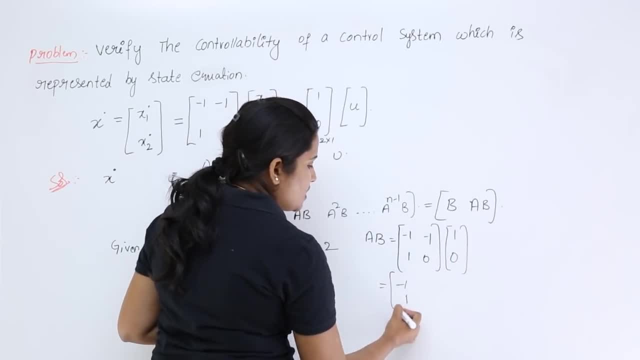 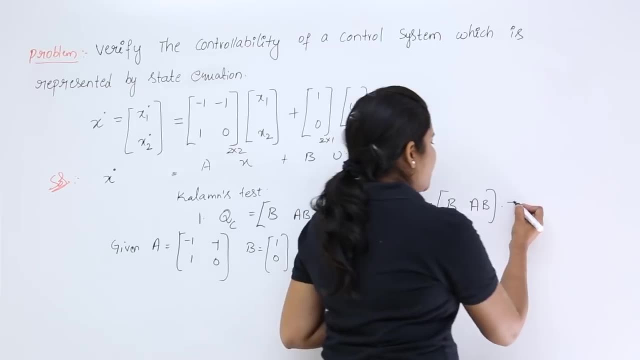 one 1 into 1, 1, plus 0 into 0, 0.. So A- B, you will get minus 1, 1 and already you are having B, So that is 1, 0. I am taking directly, So this matrix will be equivalent to B means. 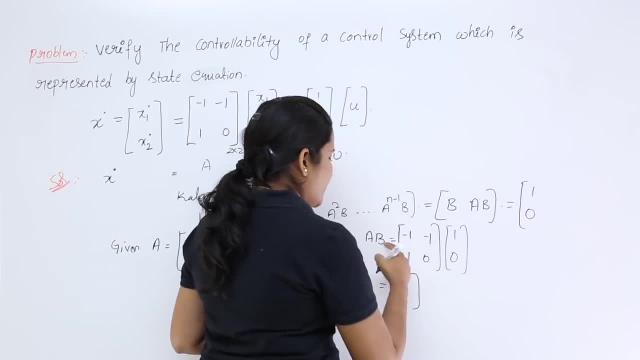 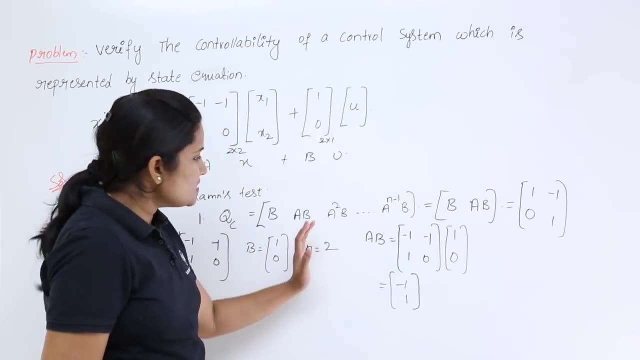 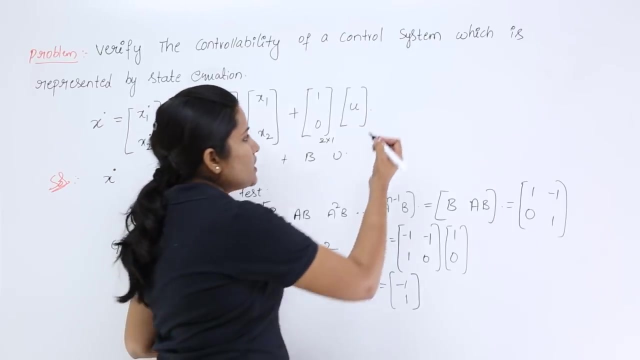 1, 0, and here A, B means minus 1, 1.. This is the QC matrix. If formed the QC matrix, the second columns test will be taking determinant of the QC matrix. So now the second step in columns test. 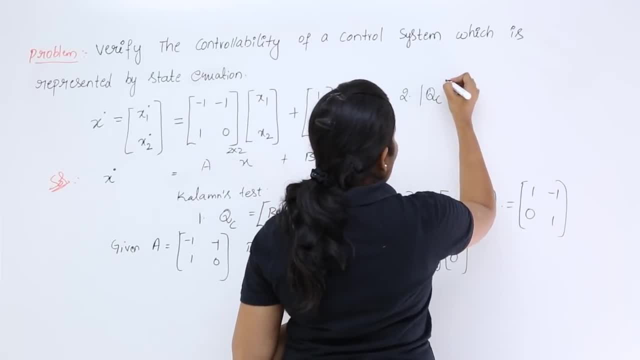 is to take determinant of QC. So if you are taking more or less of QC, then you need to take minus 1, 1, 0.. So if you are taking more or less of QC, then you need to take minus 1, 1, 0,.